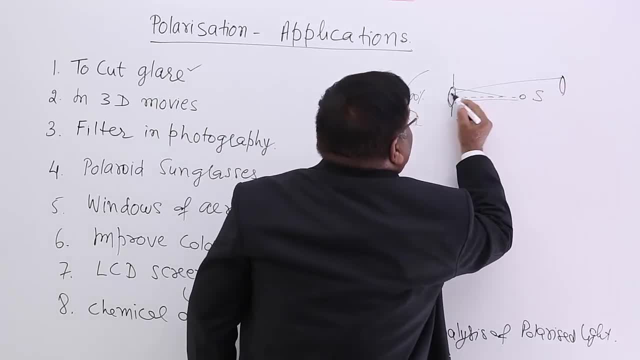 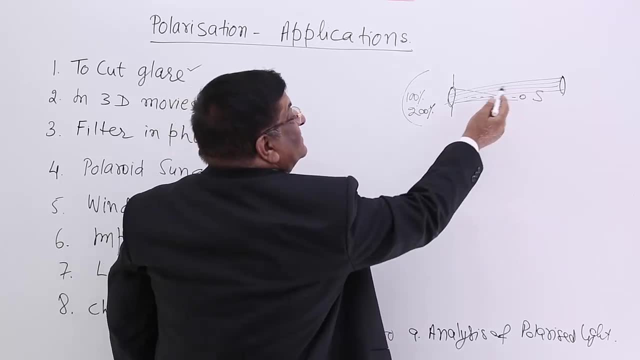 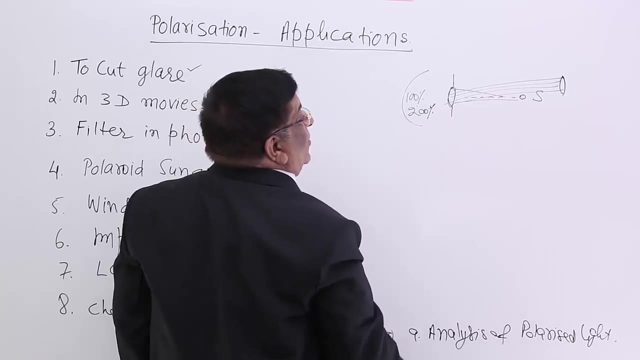 suddenly a car comes here. if a car comes here, lot of light comes here, and now this light has become 200%. if the light has become 200% and retina cannot bear it, it will get damaged. what is the damage control? it immediately ask this pupil to decrease its size. so this: 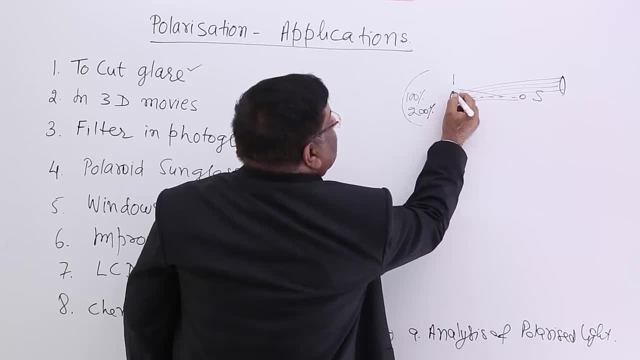 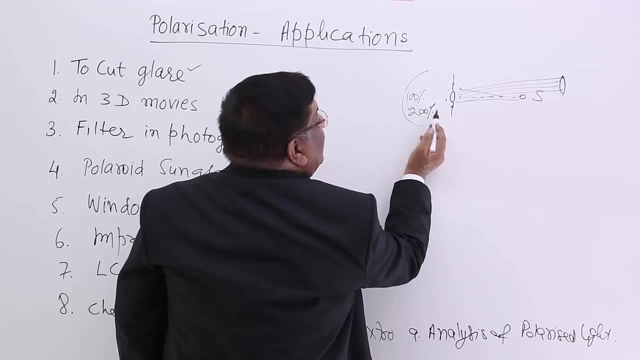 window now decrease to half. this much it become. it was so large, it has become small. so this light which is coming 200, now this also become 100 and we can see the car head light, but this size has become small. when this size has become small from the cycle, this light 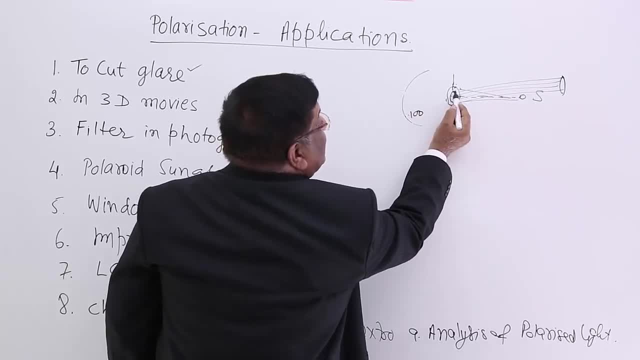 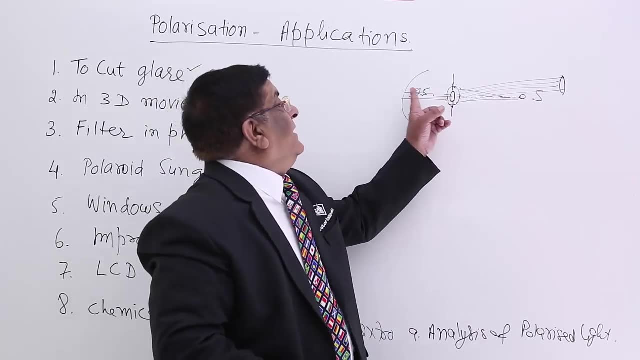 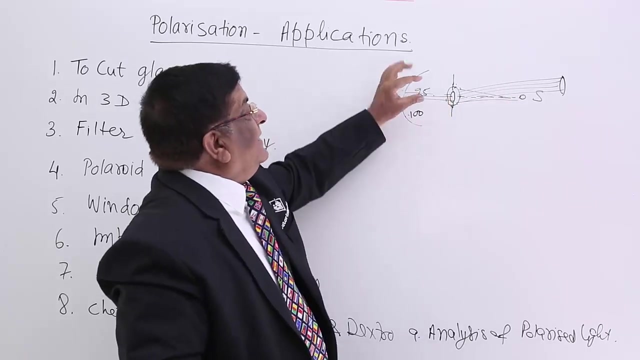 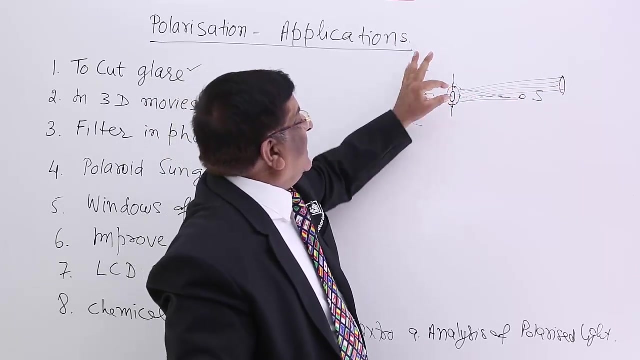 which was coming to the large size as 100 rays with the small size. now it can come on only 25. 25 is not acceptable to the eye. what it needs 100. earlier cycle was showing 100 because the size was large because of the light from the car. it has to reduce its size. 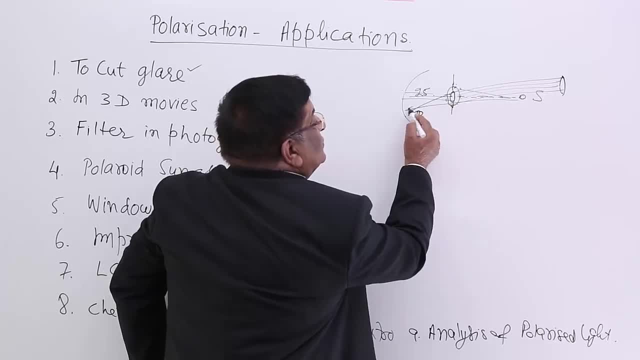 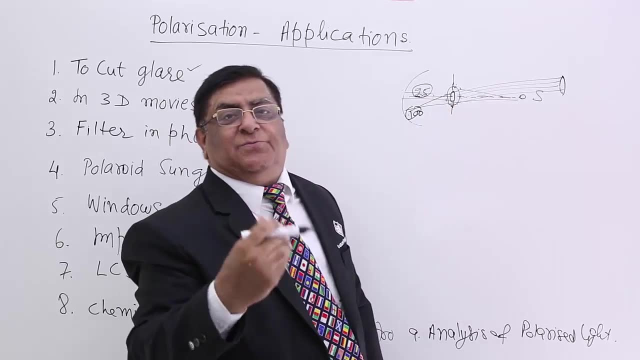 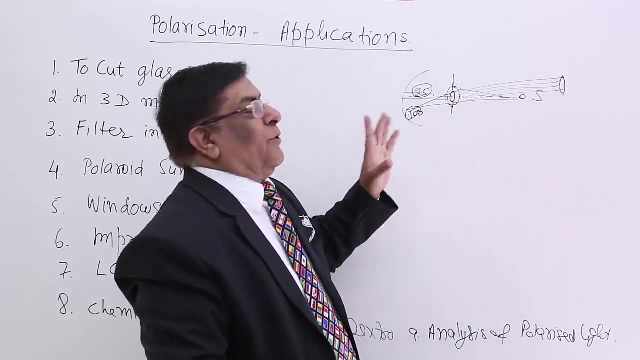 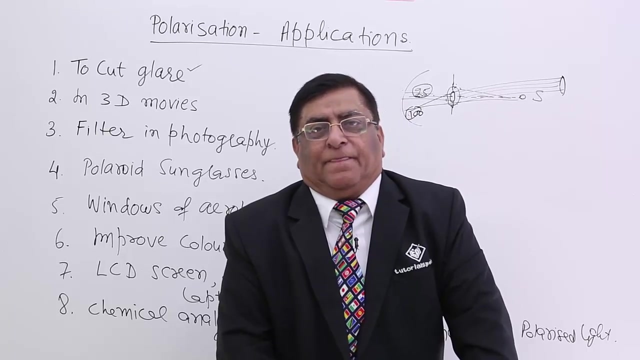 to make the car light as 100. so with the reduced size the light from the cycle has reduced to 25. so cycle is not visible. and we go and hit the cycle and we say what was the problem? the glare of the car was the problem. this is the problem. this is called glare. then how polaroid helps it. see at the 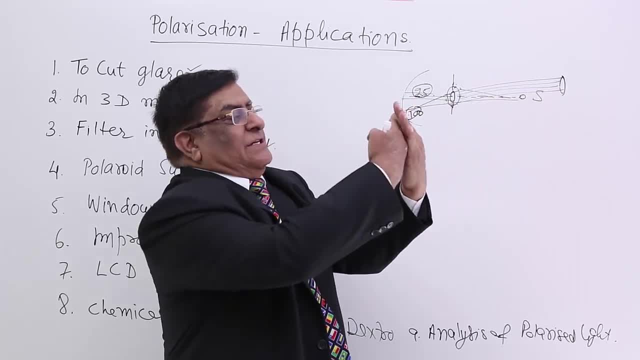 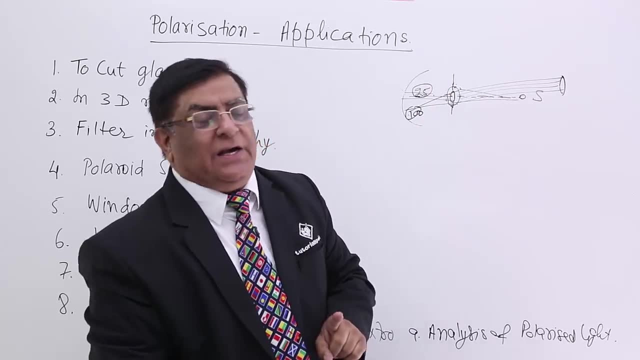 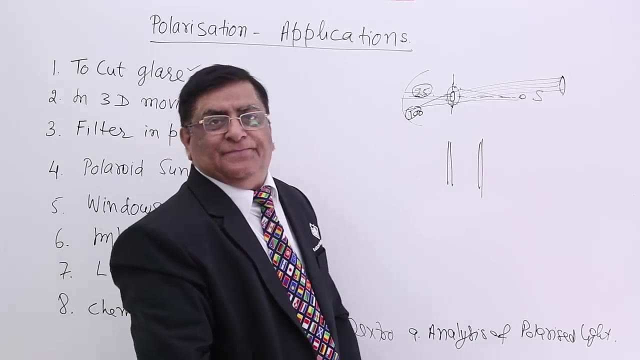 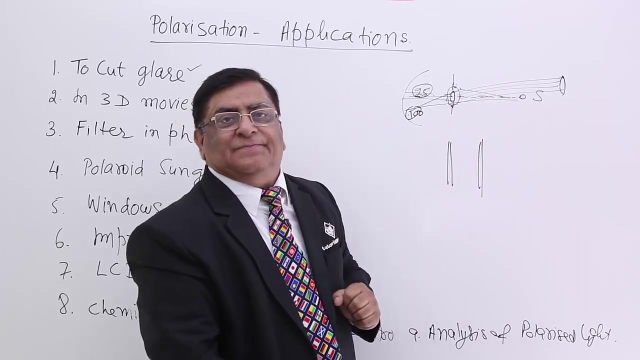 car. when the light comes, there are both vibrations: this vibration and this vibration on the headlight of the car. on the headlight of the car, we use this type of polaroids, vertical polaroids. so which light is now coming? answer: vertical light is coming to our eyes. 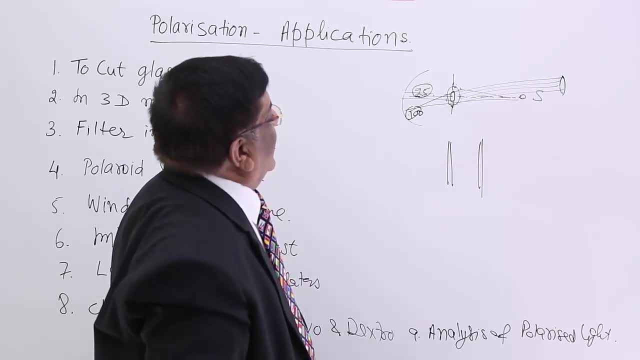 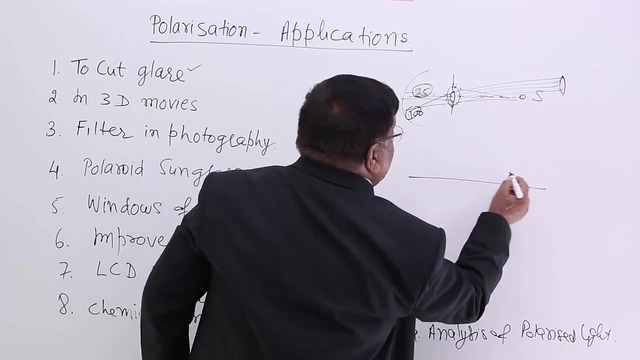 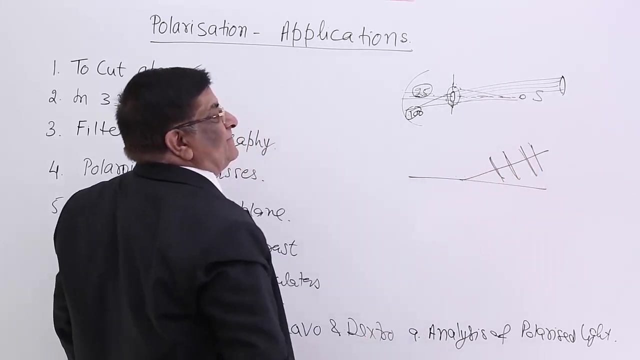 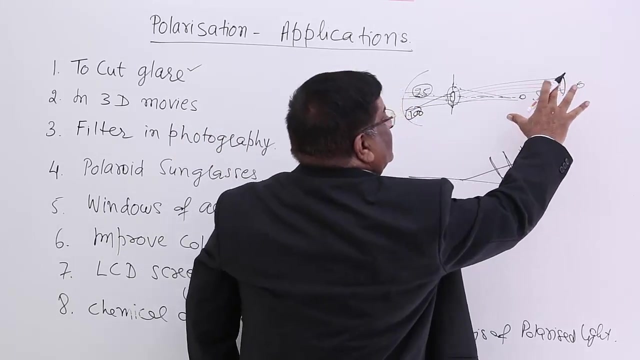 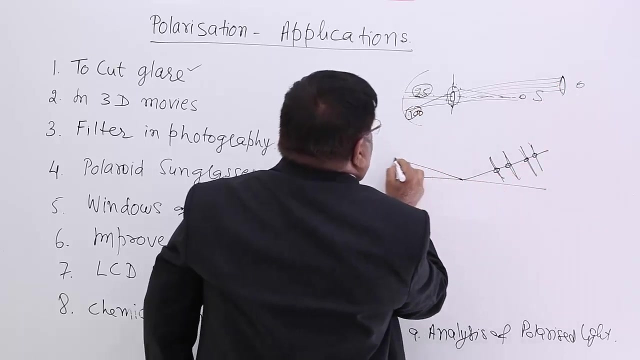 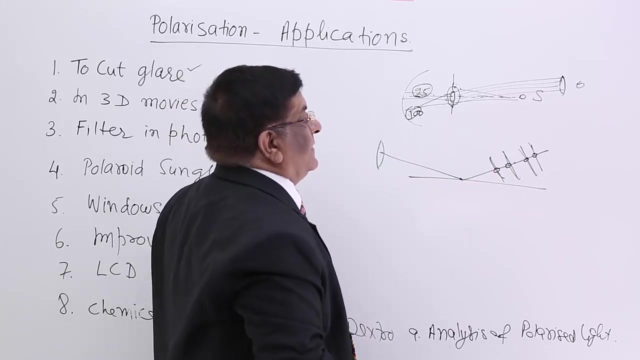 ok, these vertical lights are coming to our eyes, yes, and when this vertical lights fall on the ground, this what will happen? this will get absorbed. sorry, let me put it other way from here. the light has got both. the vertical one is absorbed on the road and it reached my eyes. then the intensity has become half, why i have used polaroid. 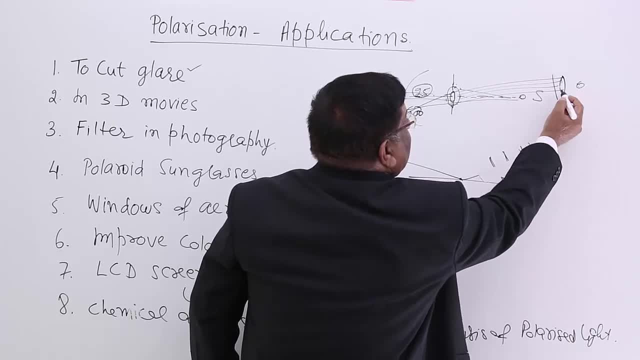 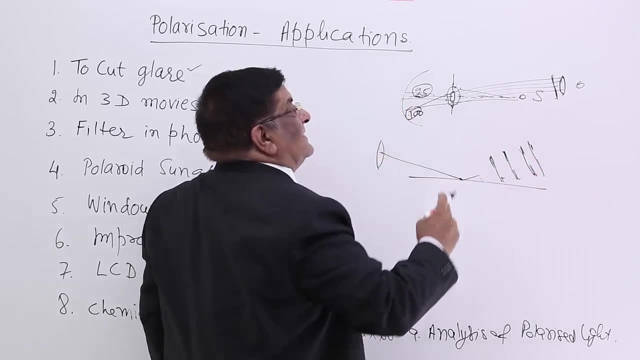 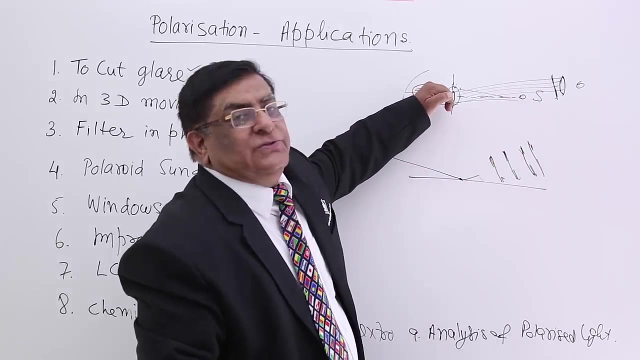 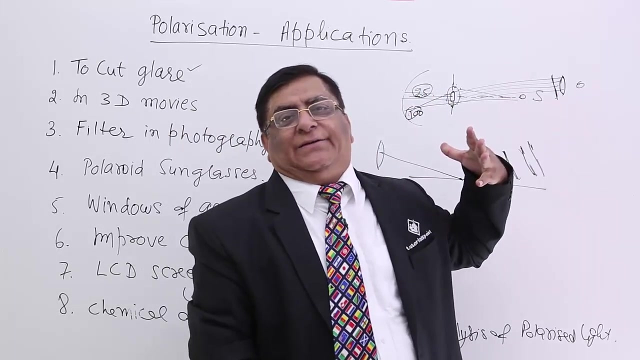 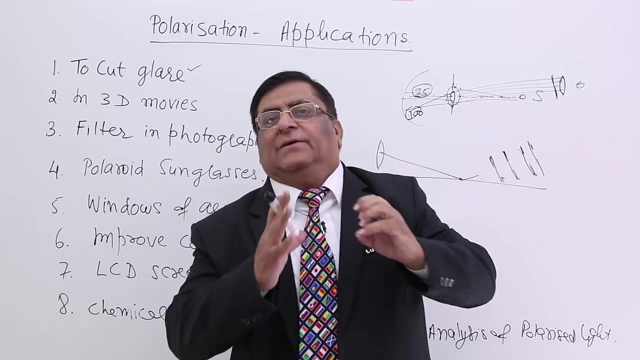 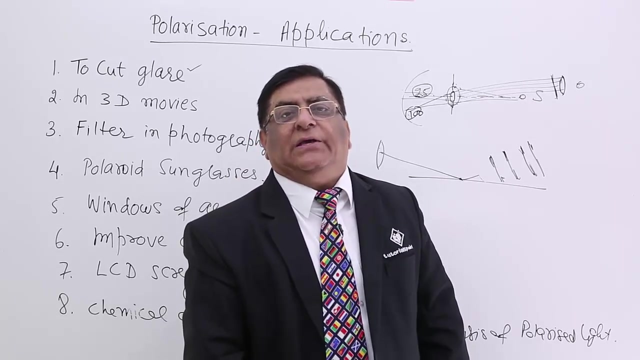 here from the headlight of the car. I am using the polaroid and because of this polaroid the intensity becomes half. when that intensity becomes half, then this effect also decreases, so then I am not having the glare. so this polaroid material used before the head light, that is sufficient to show him the ground why it gives only one. 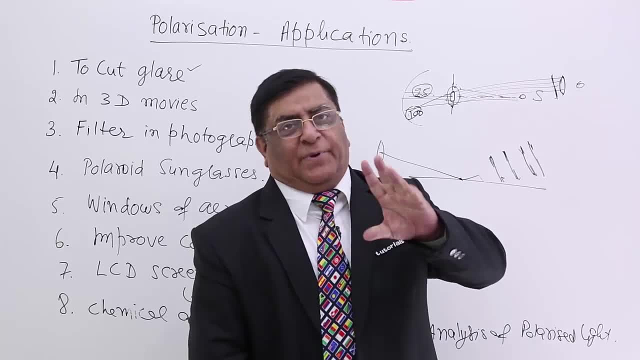 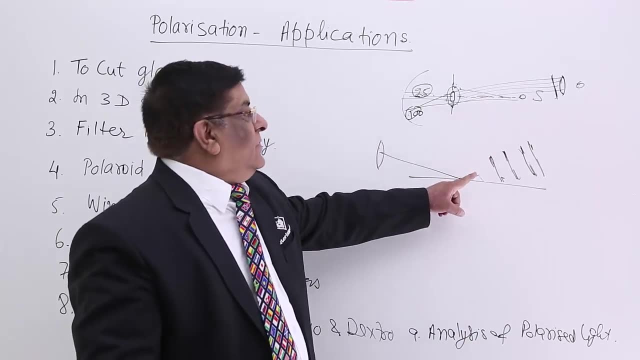 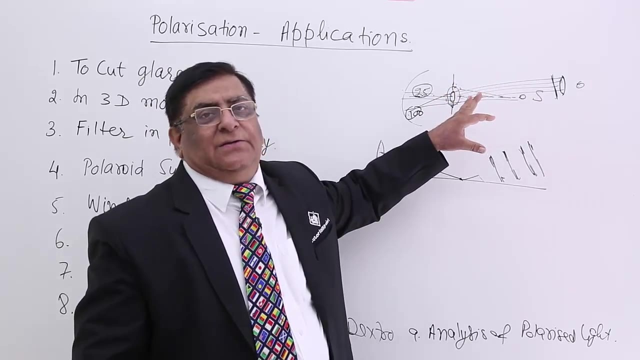 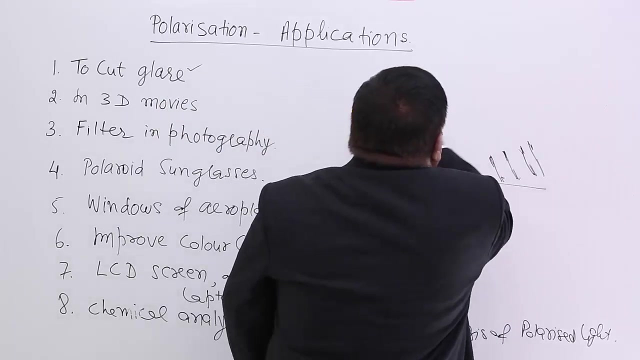 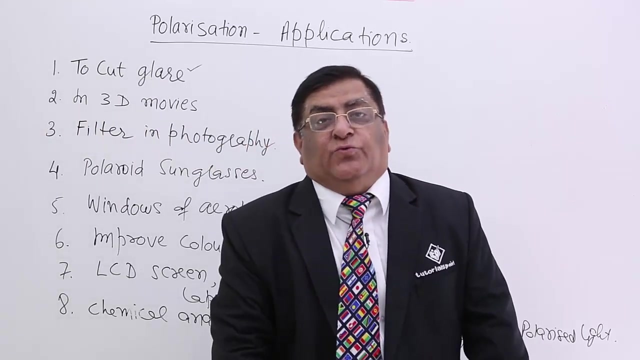 direction of the vibrations. okay, so this one type of vibrations are cancelled. therefore we get less light, less intensity of light, because it has less light has become polarized. So that is how we can cut the glare of the car. Now the second thing is in 3D movies, In 3 dimensional movies. it is a long technique for 3D movies we have. 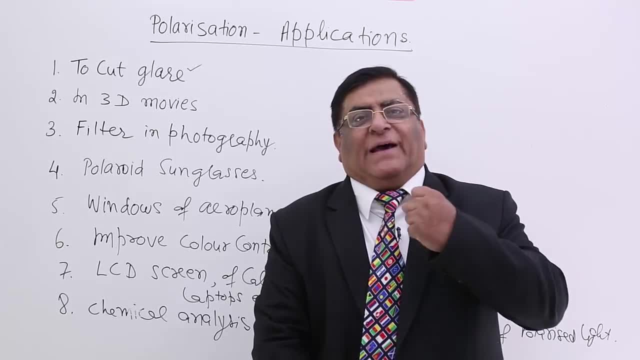 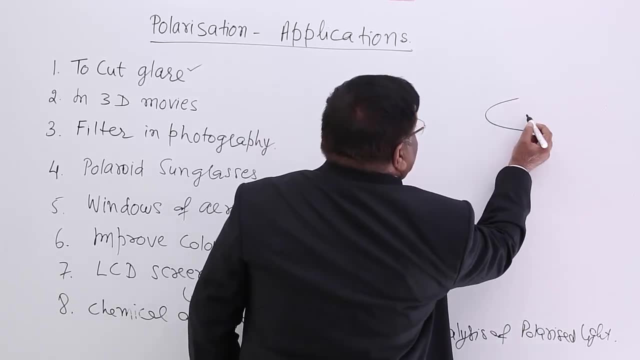 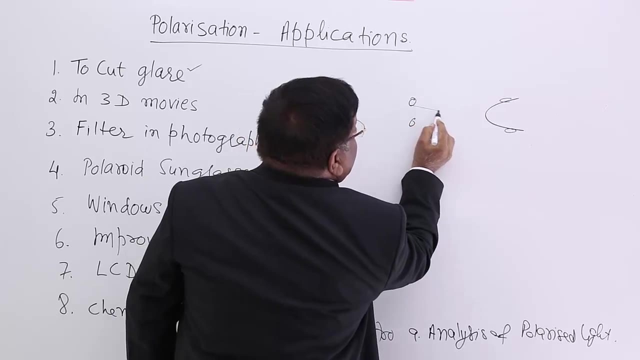 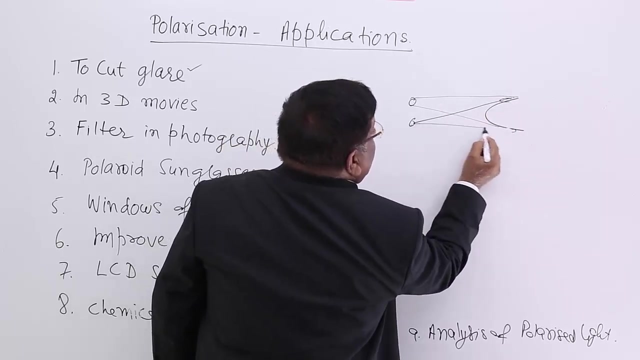 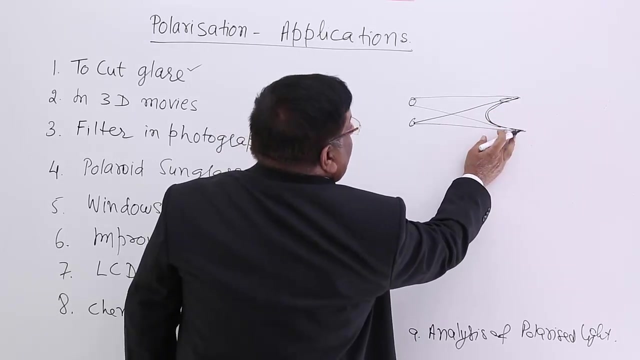 to see, we have to replicate the method of seeing with 2 eyes. How do we see with 2 eyes? If I am seeing this face from 2 eyes, then this eye looks this portion of the face and this eye looks this portion of the face. This portion is different, then this eye looks. 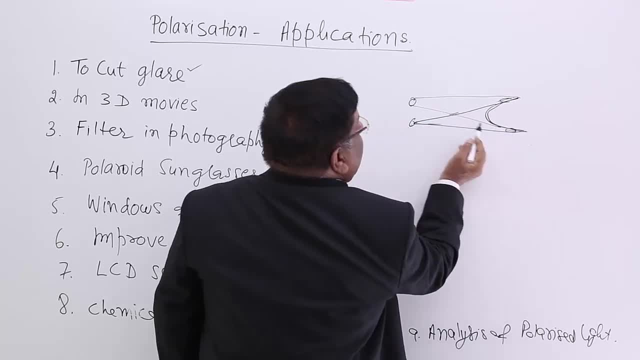 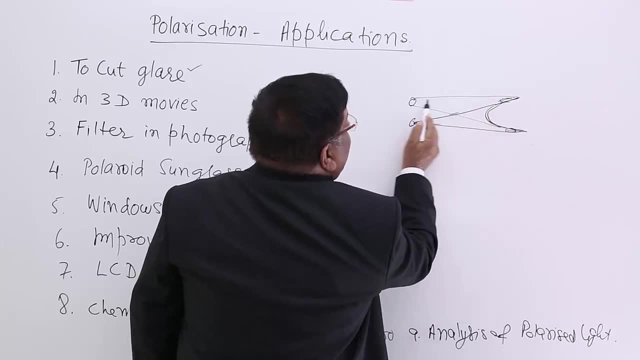 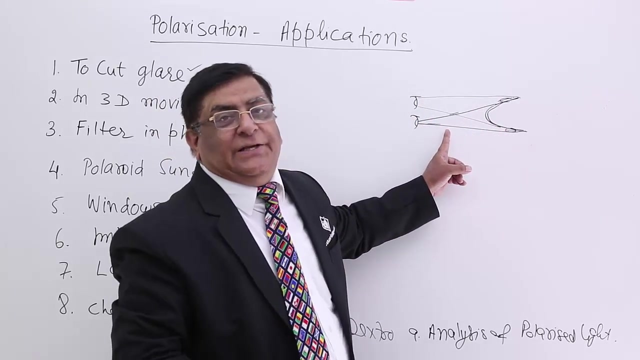 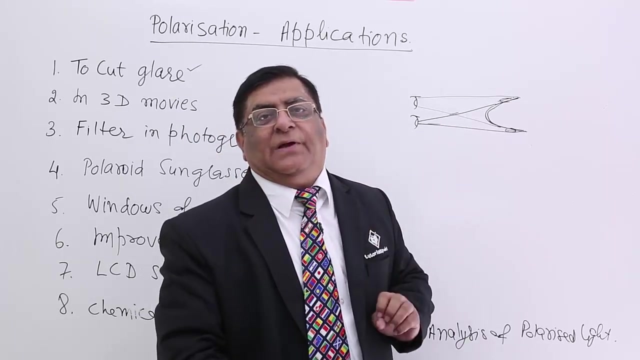 this and this, You see, this eye can look this ear, this eye can look this ear. this cannot see this ear and this eye cannot see this ear. So these are our 2 eyes. So there are 2 different images made by the 2 eyes. These 2 images are sent to brain. brain process them And here you 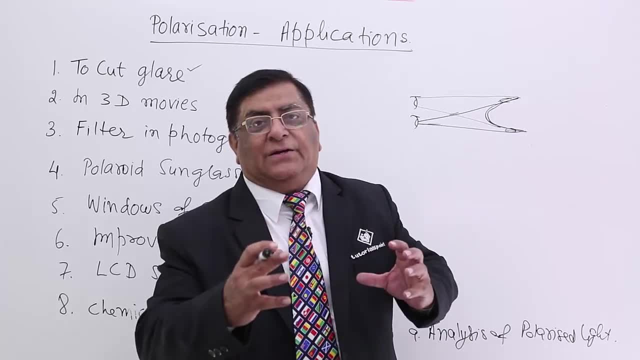 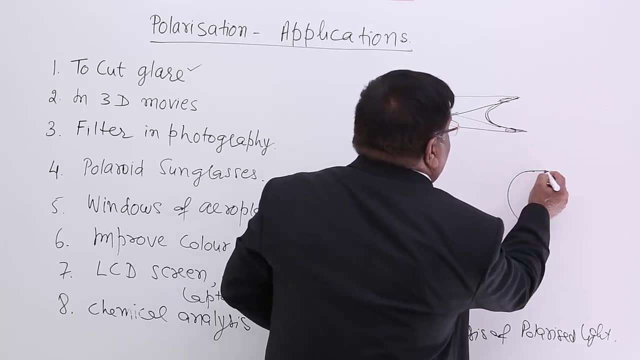 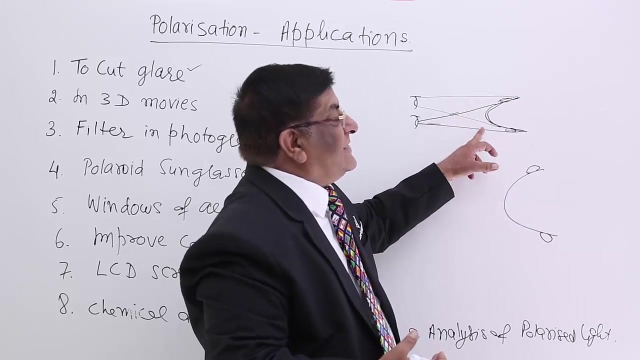 see, he makes a figure, 3 dimensional figure, And he is able to make this figure, whatever it was, the original shape. he make that original shape. That is a sculpture. He is able to make a 3 dimensional sculpture With help of these 2 images because they were taken. 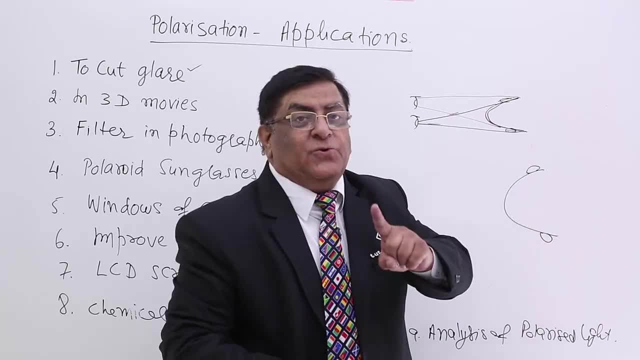 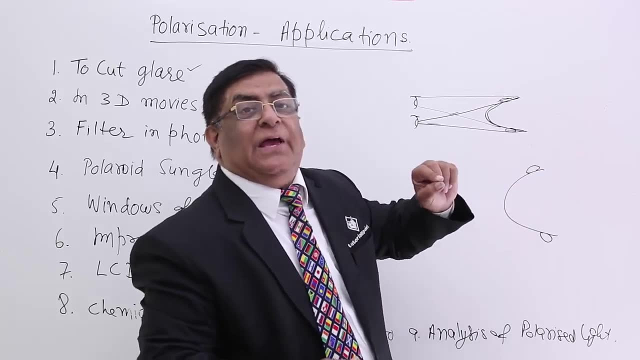 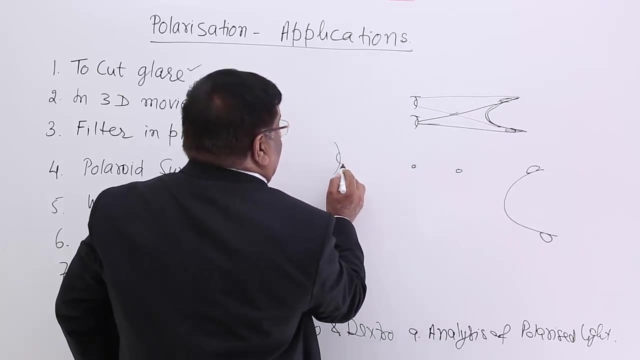 from the different angles. ANCHOR- 1, 2., 3.. If you see from one angle, you will not be able to measure the depth of any material. These are the two points. If I see it from here, I cannot say which is in front and which is in the back. 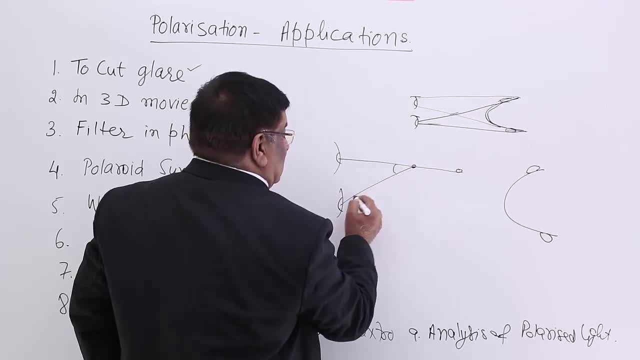 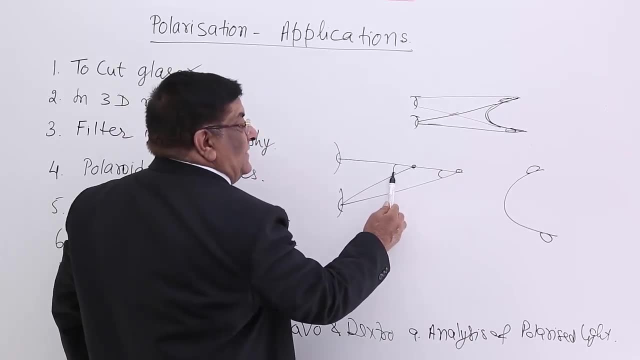 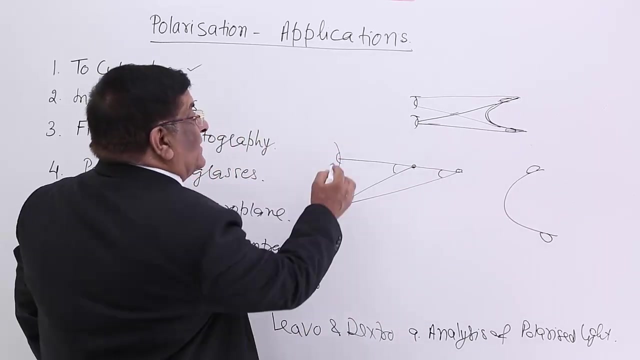 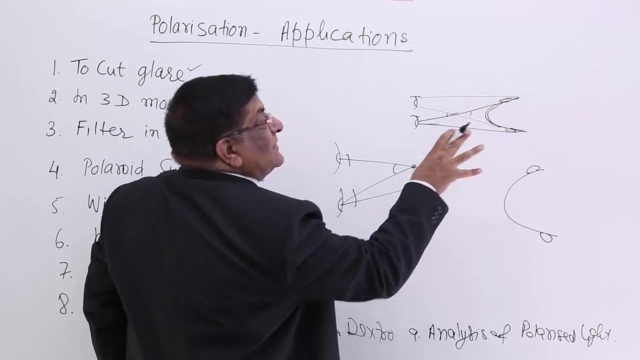 If we have another eye, then this angle is large, this angle is small, and then brain has understanding that this is in front, with the large angle, and this is on the back side, with small angle. So what is required? Two pictures are required, and this angle decides the depth of any particular material. 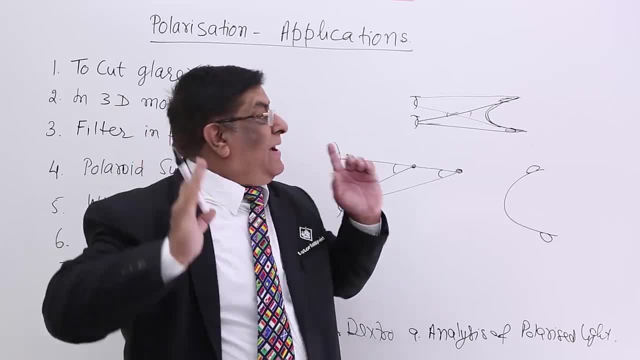 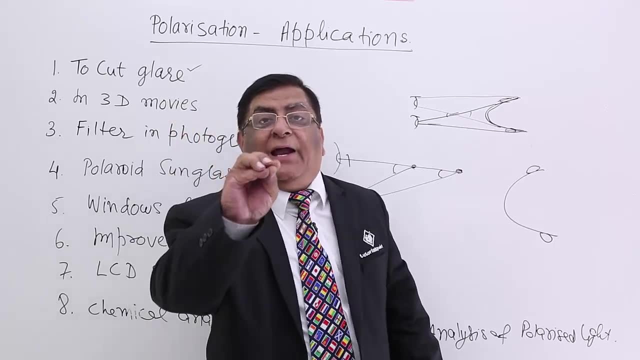 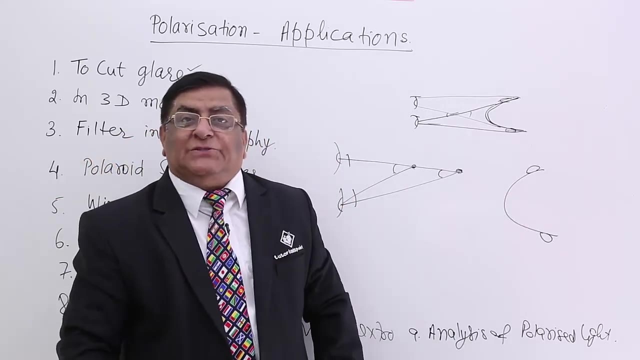 So depth made by our ears, Angle made by our ears, is always less than the angle made by our nose. If I put my hand this way, it is making bigger and bigger angle to you. That is why you see that it is coming closer to you and you are using both the eyes. 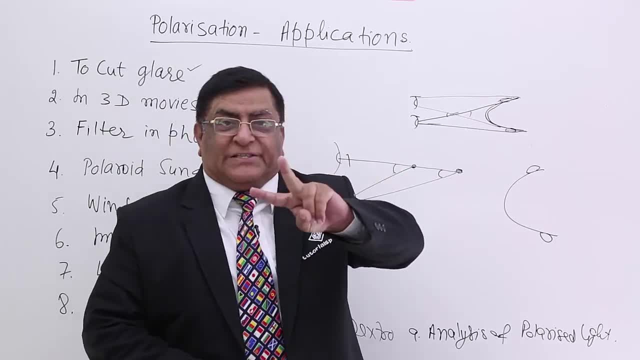 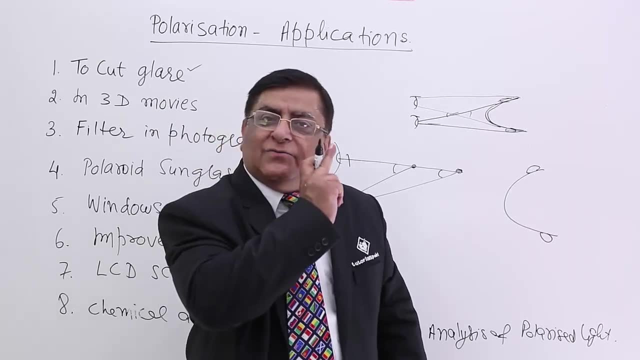 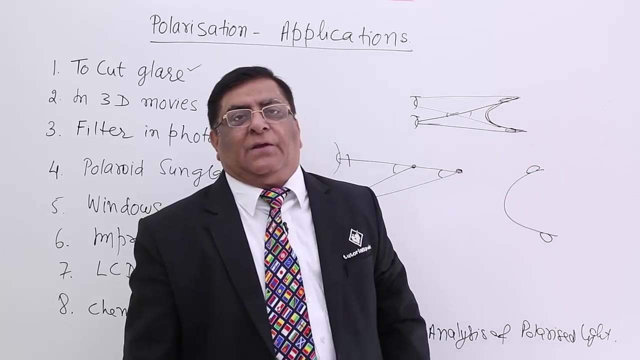 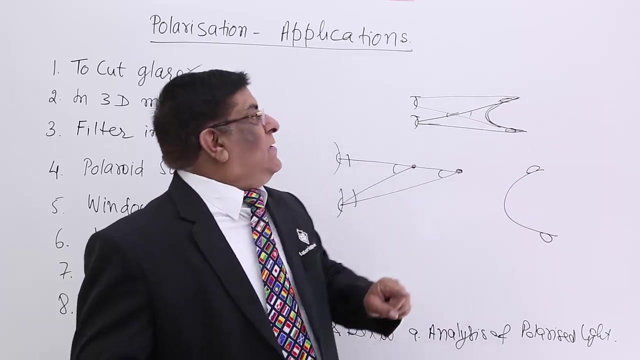 Now. so we need two pictures, two separate pictures. One is visible by this side and other visible by this side, but unfortunately screen before us is only one. So we have developed a technique: On that screen we project two pictures. 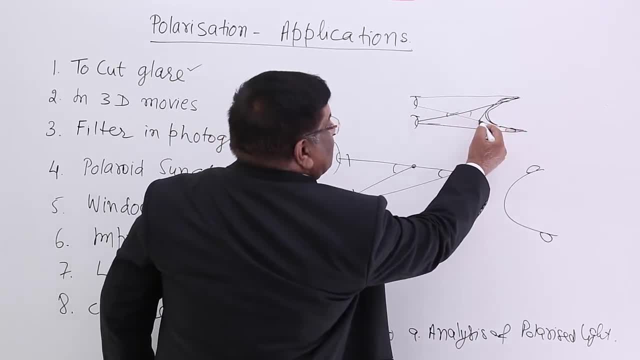 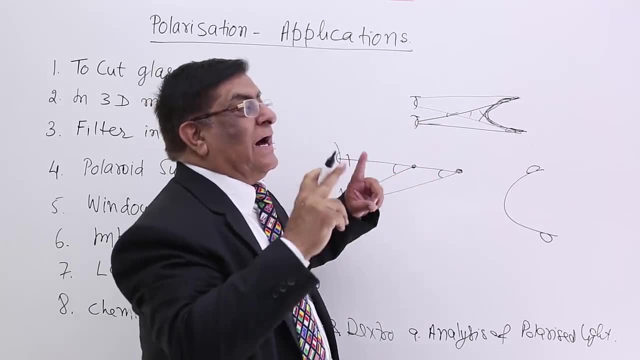 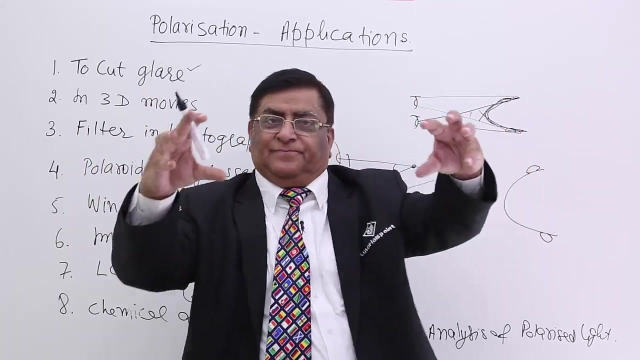 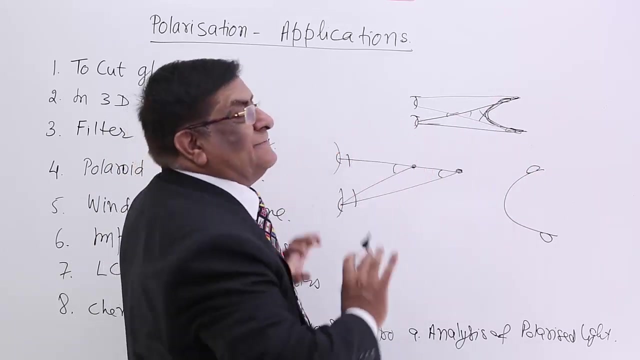 One picture which camera is taking from this side, other picture which other camera is taking from this side. Both pictures are taken by two cameras, 1 from this side, 1 from this side. Then both these pictures are projected on the screen together. 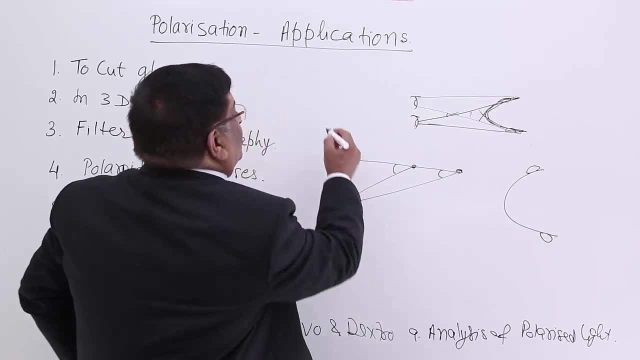 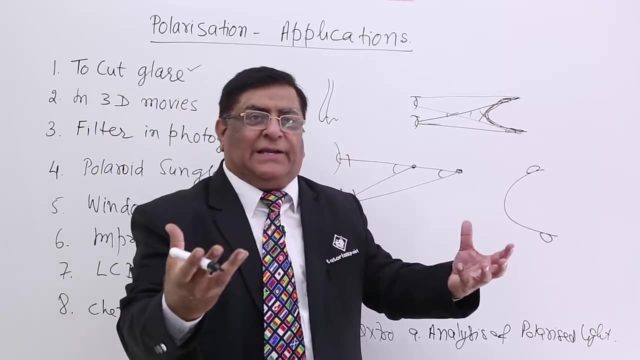 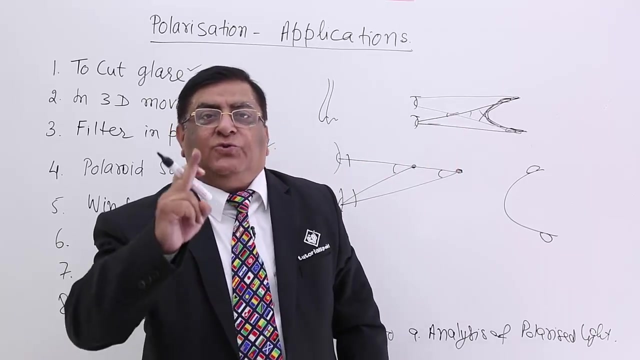 When you project these two together: in one picture you find the nose is here. in the other picture, you find the nose is here slightly different. it has to be because the cameras are at different angles. ok, Now we have to show to the brain two images separately. 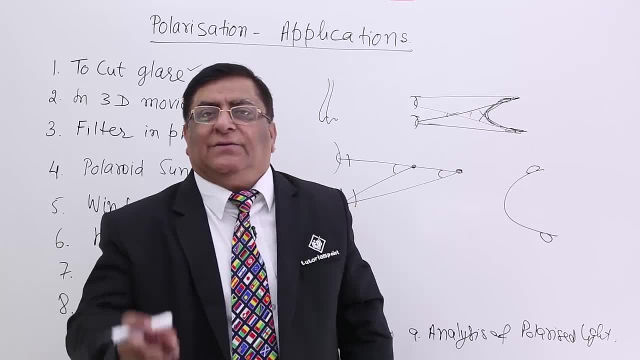 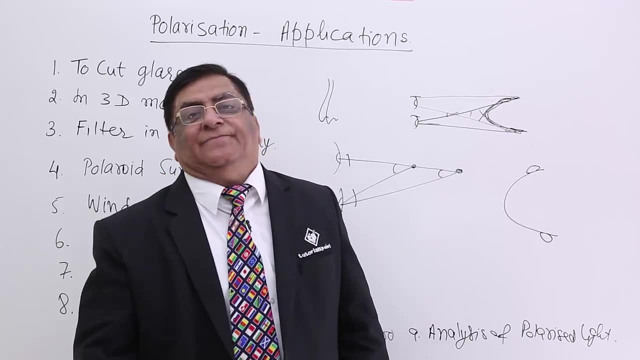 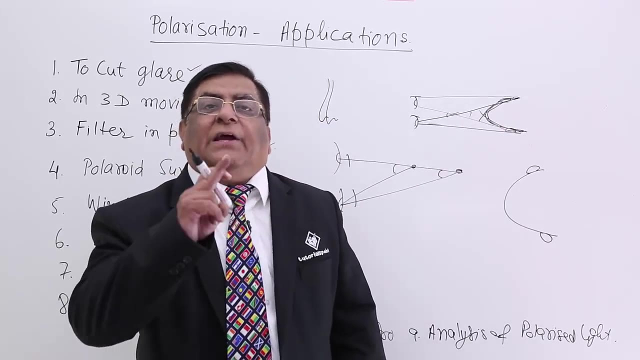 So that this eye sends one picture, this eye sends another picture and this eye should not send the picture which is seen by this eye and this eye should not send the picture which is seen by this eye. How we can do that Here? we can do it by Polaroids. 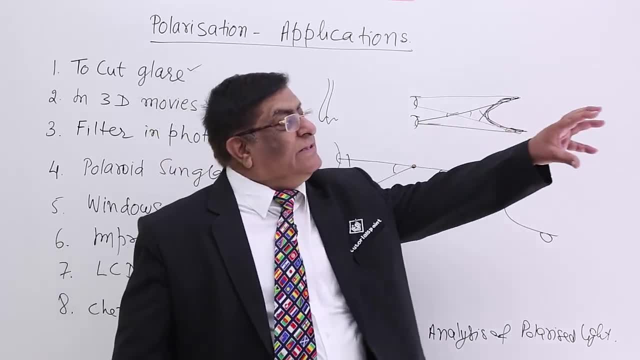 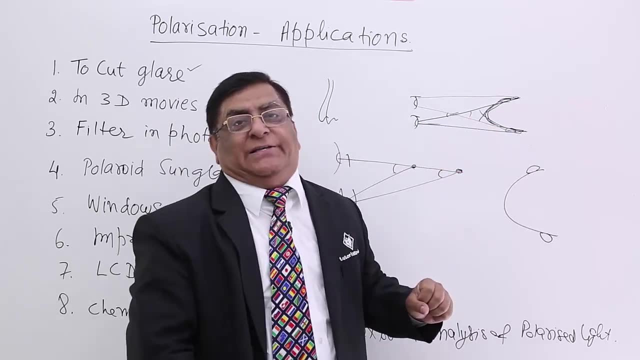 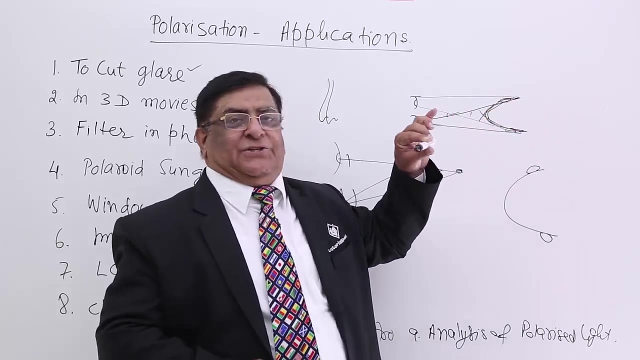 How can we do it? by Polaroids, The one shooting, The one shooting with this camera, is done by ordinary rays and this one shooting is done by extraordinary rays, Ordinary rays which have vibration. like this: All the light is polarized light, this vibration, and this camera, all the light which has got. 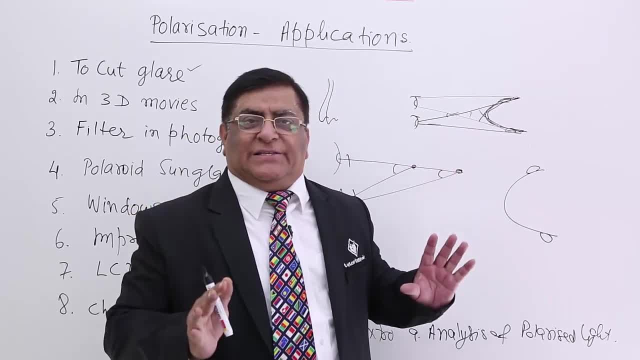 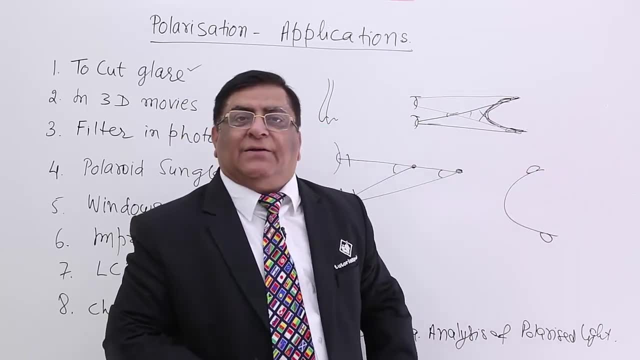 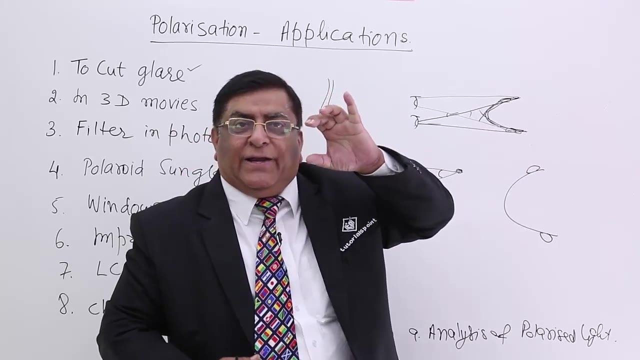 this vibration. ok, Both are making images, both images we put there In our eyes. we can see both the images. But when we have that Polaroid glass, this Polaroid glass has a Polaroid which allows only this rays. It will not allow this rays. 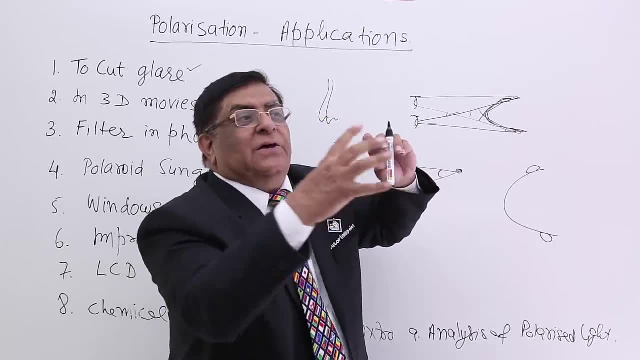 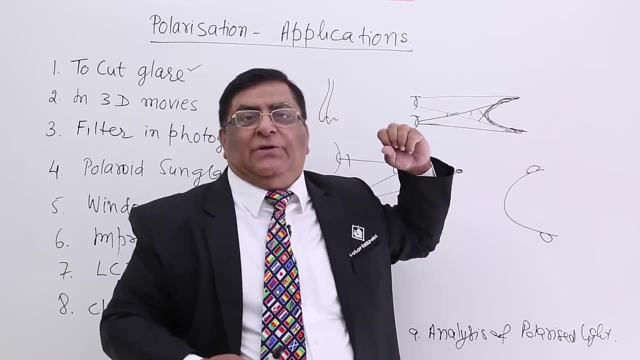 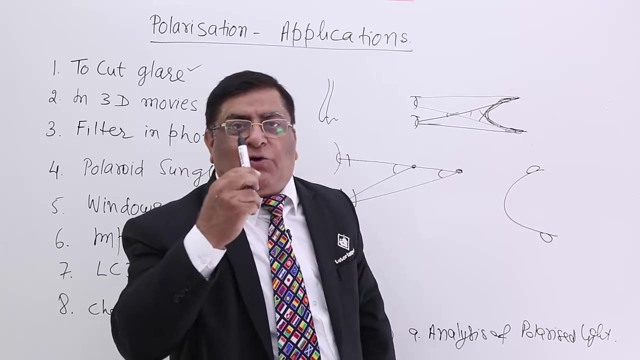 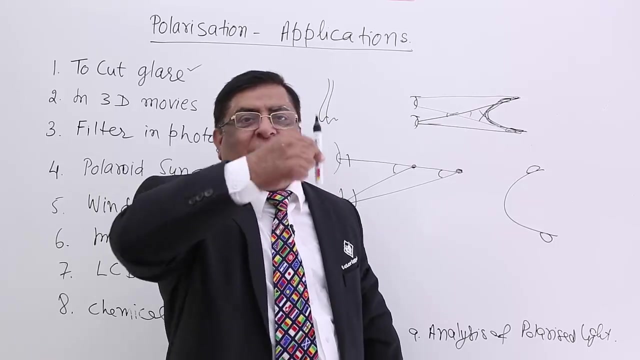 So what will happen If it does not allow? this way, the photograph of this camera is not visible to this eye. This is seeing only one image which is in this light. Similarly, This Glass Has Got System Which will show, which will allow only extraordinary or this vertical vibrations. 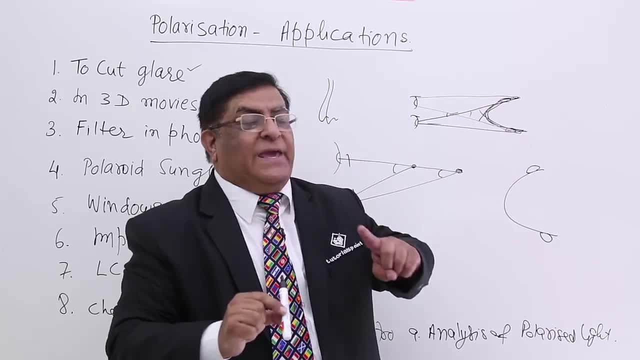 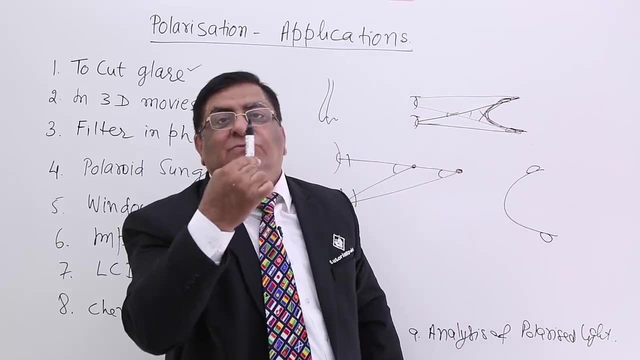 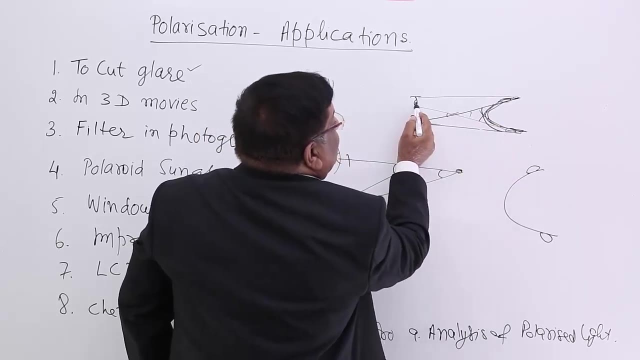 This will not allow this vibration. So the image of this camera, which was done in this vibration, is not allowed by this glass. So this will see only one image. Which image? This will see this image, This one, And this glass is seeing only this image. 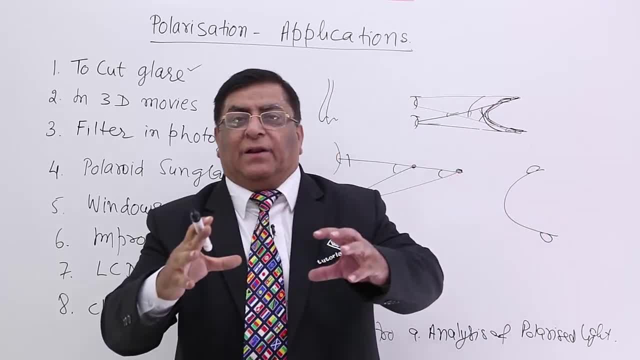 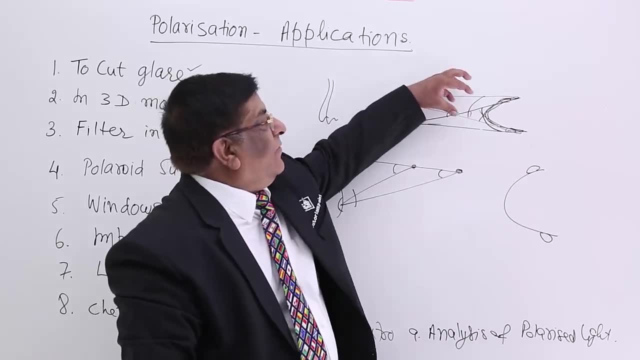 So this is the image. This is the image. Now, this is comparable as how we see the things like. How we see the things like One eye from this side, One eye from this side. This is not seeing this. This is not seeing this. 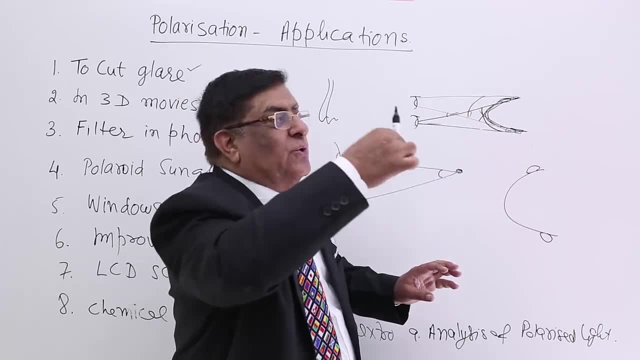 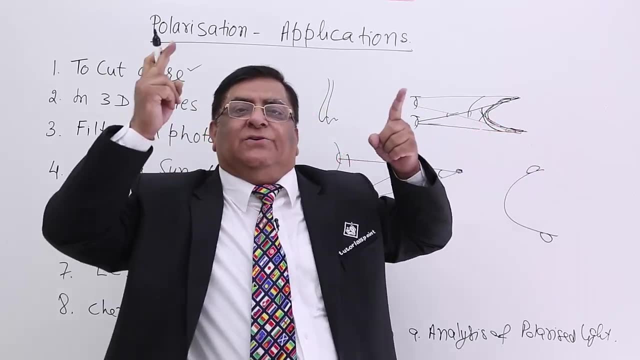 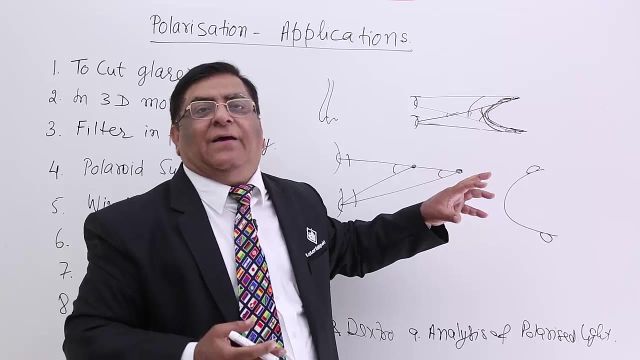 That we have created. by cancelling This will show only this side of picture. This will show only this side of picture. So both images are sent to brain And brain make a sculpture of that And he makes a three dimensional figure of that. 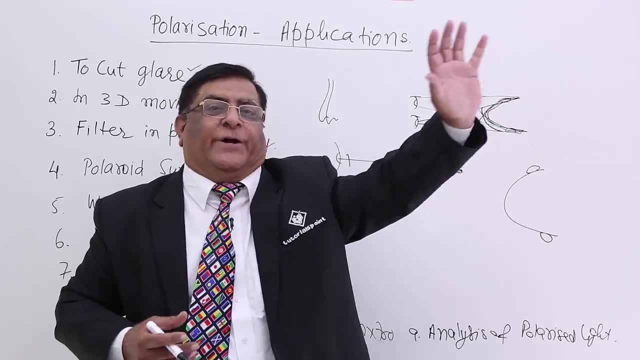 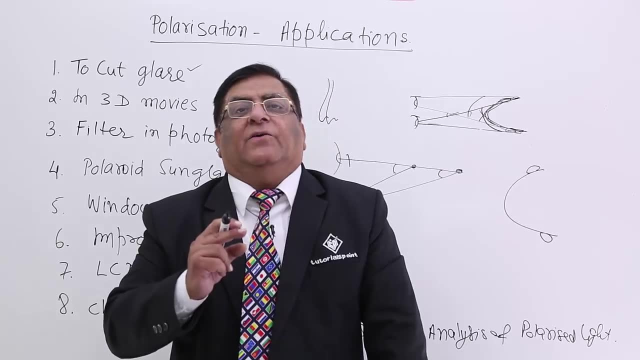 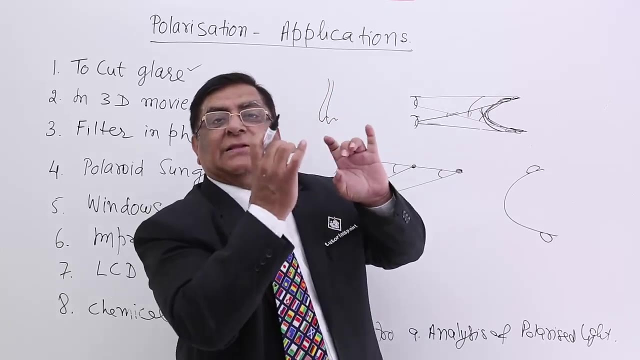 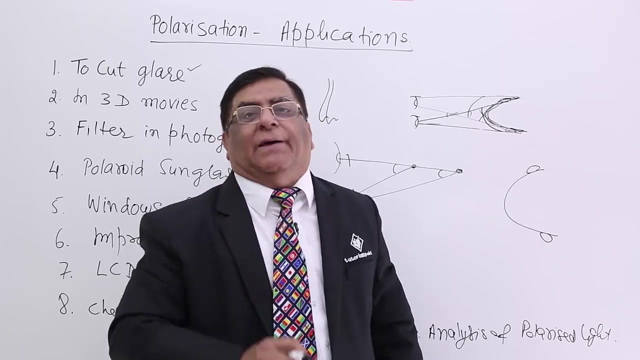 And it appears to as if somebody is lying before us. Here we have used polaroids when we are photographing. Here we. polarized light is used in photography And we have used polaroids to filter them when we are seeing the picture. That is why in all your 3D TVs you have the goggles with them. 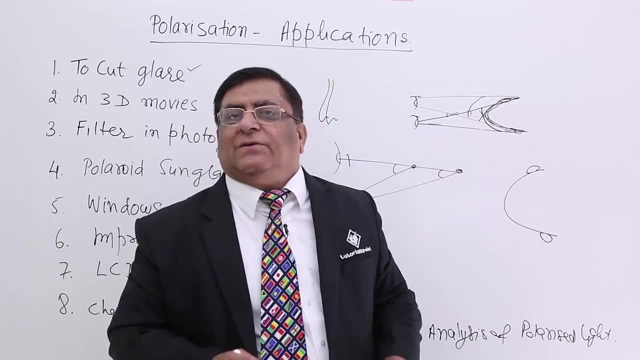 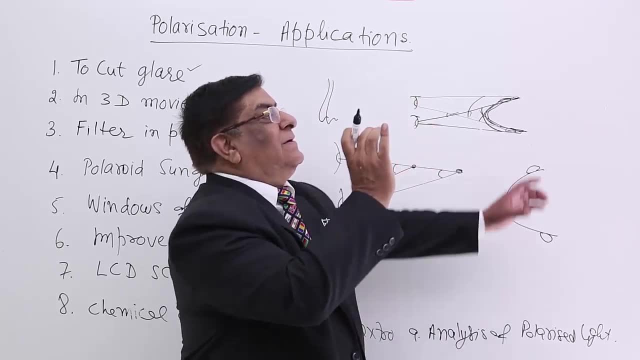 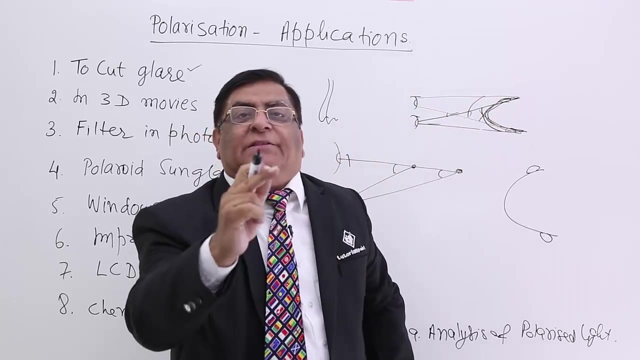 That is necessary, And this, this. You can do all the experiments with those goggles. Those are polaroid. See something in this? See, have the other goggles. You see something here And put it here, Rotate it. You will see everything what I have told you. 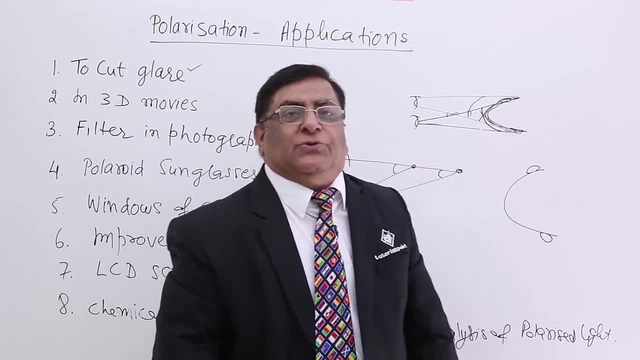 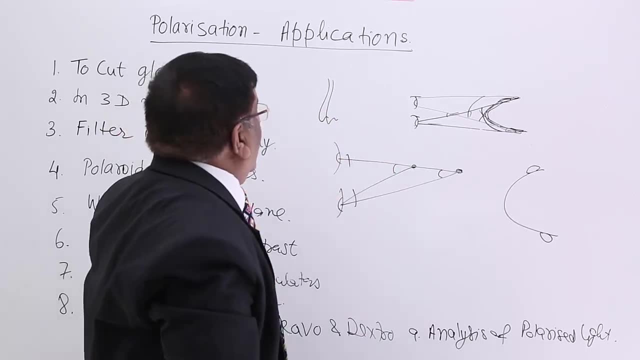 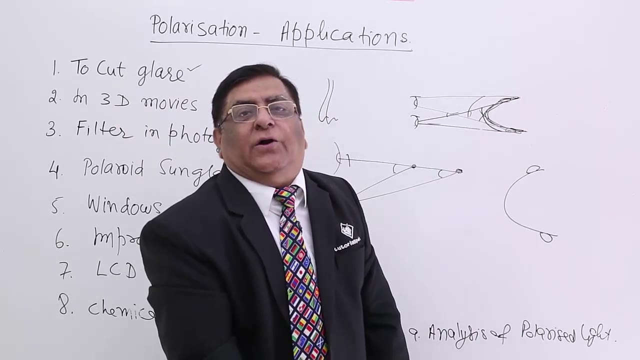 And it will be very interesting. You will find it. So next time, do it with the glasses of 3D. You will find that polarization effect. Okay Now, even if you see any reflected light with that, You can find out whether it is polarized or not. 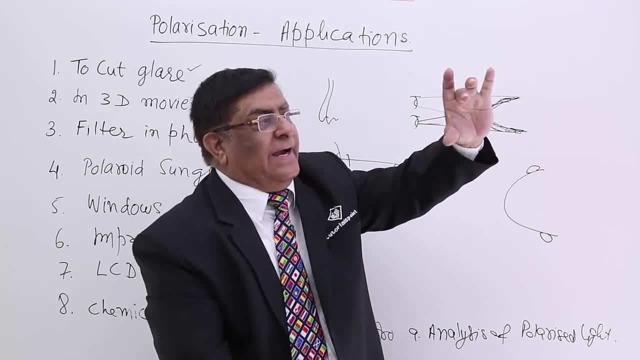 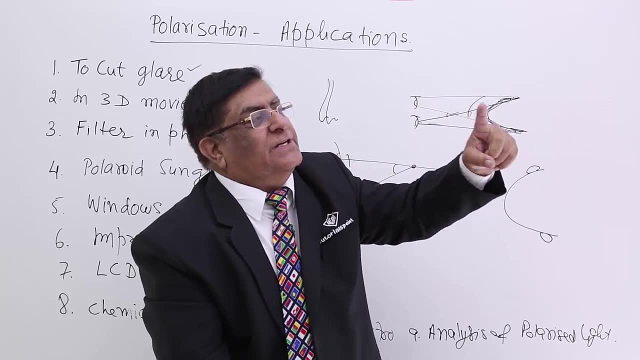 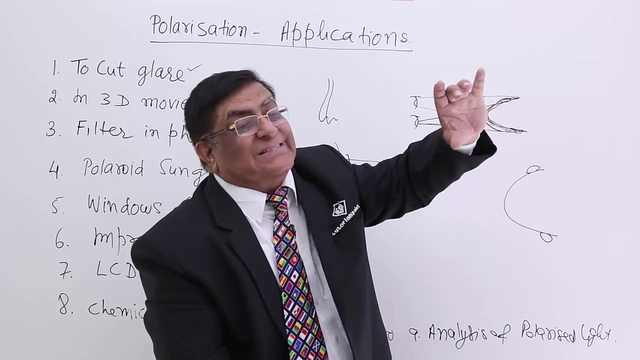 I am seeing this picture with that glass- One glass, And I rotate it. If, by rotating, the intensity of the light does not change, Then it has vibration in all the direction and it is a unpolarized light. But if, by rotating, I find the intensity is becoming less, less, less, 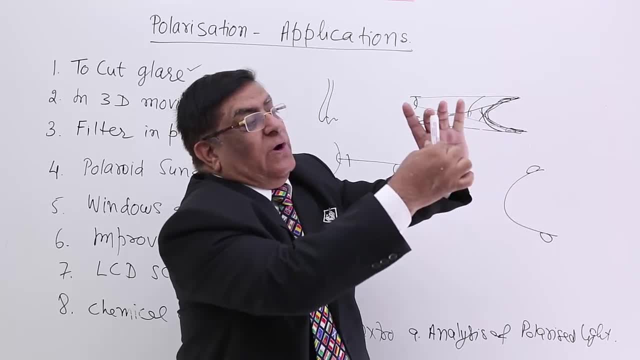 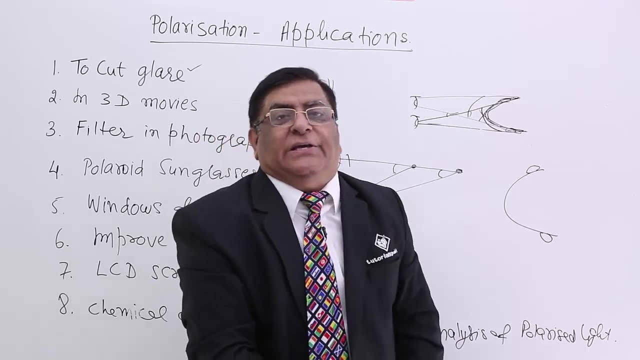 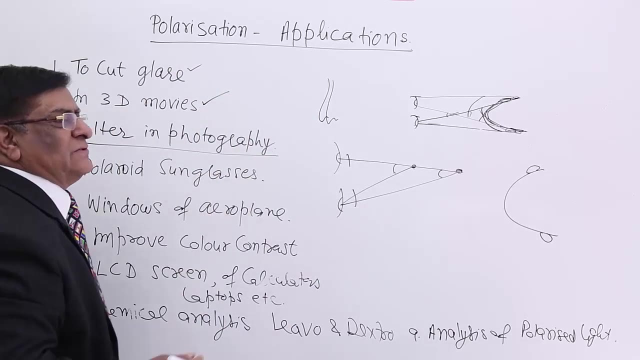 That means it is already a directional one. It shows full light, Then it shows no light, half the light. This you can see by those glasses And that is a wonderful thing in your house. So that is 3D movies. Then in the photography, same thing: we want to cut the glare. 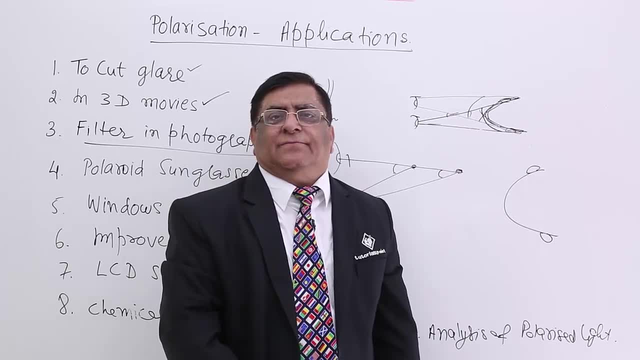 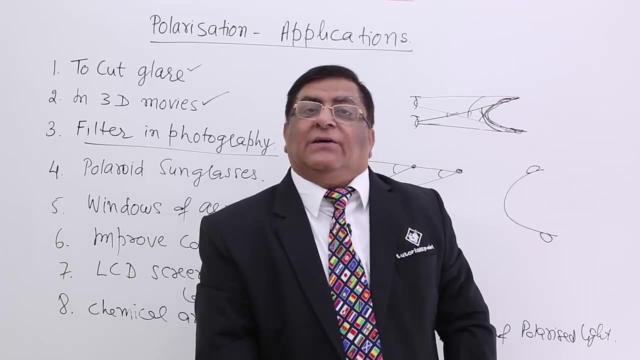 So when we do not want to change the colors and we do the photography only if sunlight is less, We cannot make the sunlight less, Nor we want to use any colors, So that color will come in the picture. We do not want color in the image. 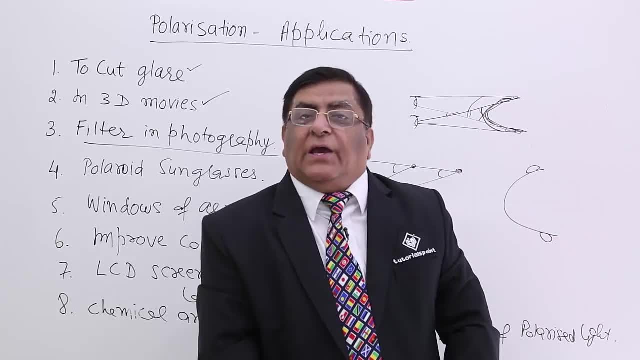 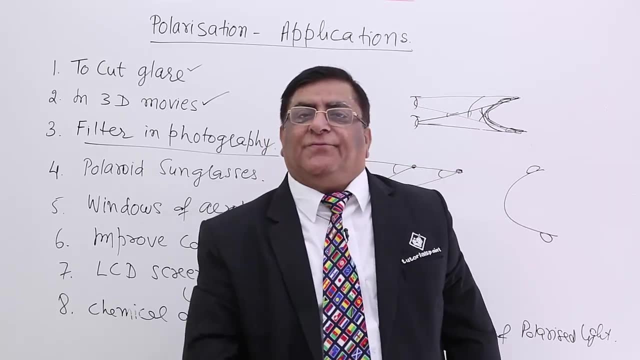 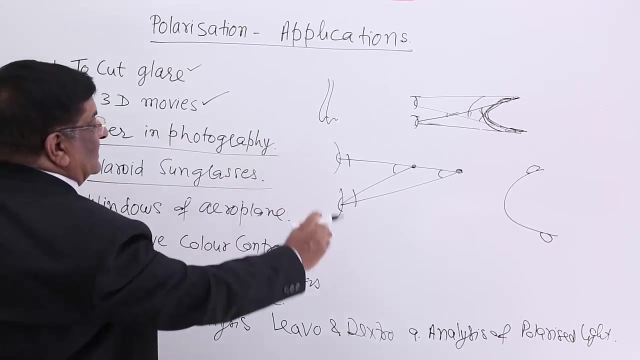 We do not want that much sun. So what we can do, We can use a polaroid which will cut one side of vibrations and intensity will become half, So we will have a beautiful picture with photography filters, Then polaroid sunglasses. Same thing for the sunglasses. 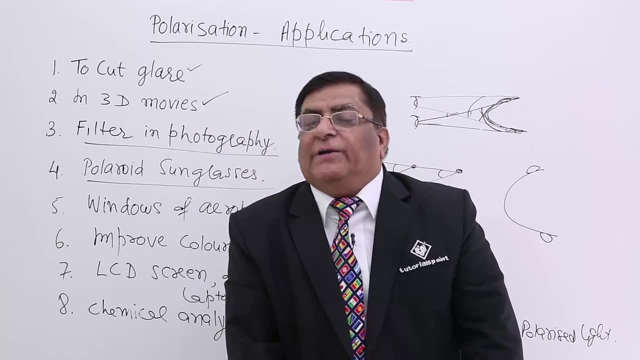 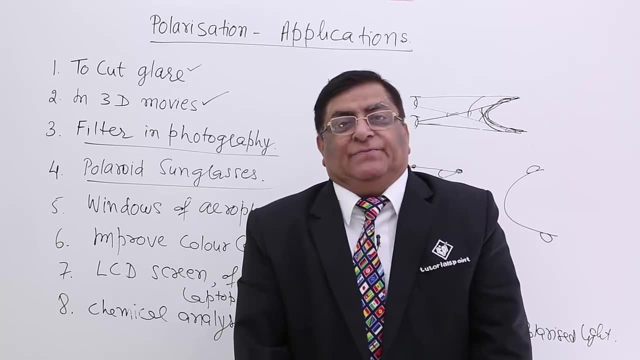 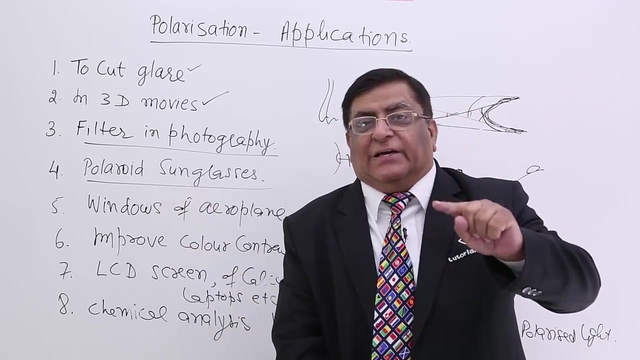 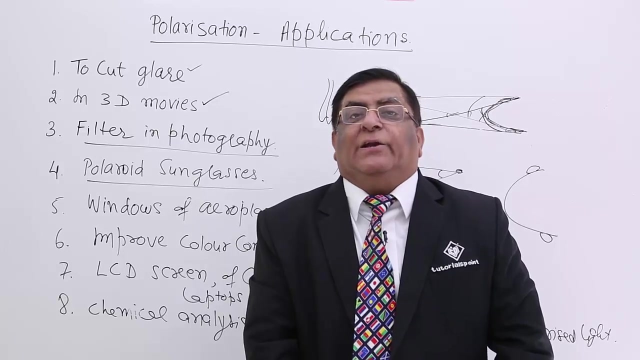 Polaroid sunglasses have a specialty That They should not decrease. I should say Yes, They should not mix up color with the image. with the ordinary glasses we use sunglasses They are mixing certain colors and they are cutting other colors. Like if I use pink glasses then it will cut the blue color of the light which is coming. 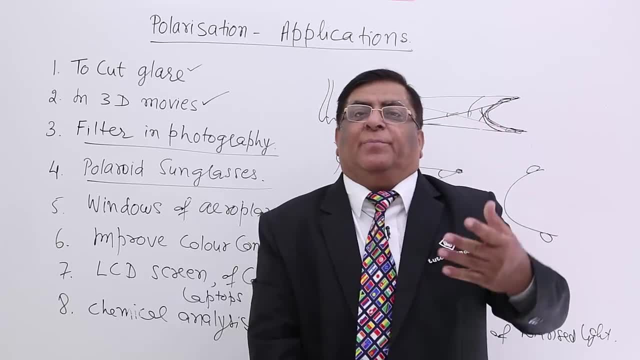 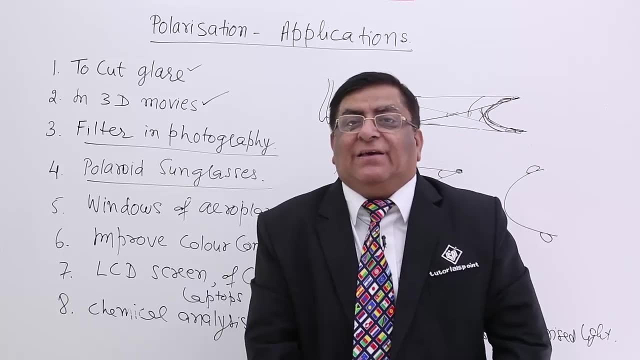 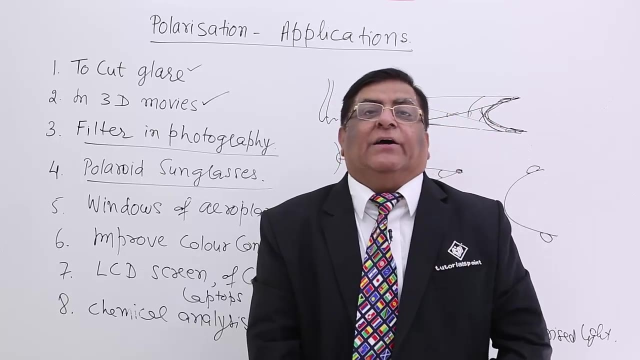 to me And anything blue I see, that will appear to me black. So that is the thing, Thank you. If I have blue glasses, gray glasses, blue glasses and I see a rose, the rose will look black because it will allow blue color. it does not allow red color to come. 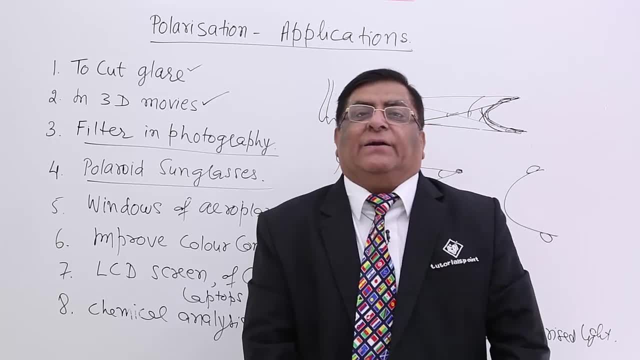 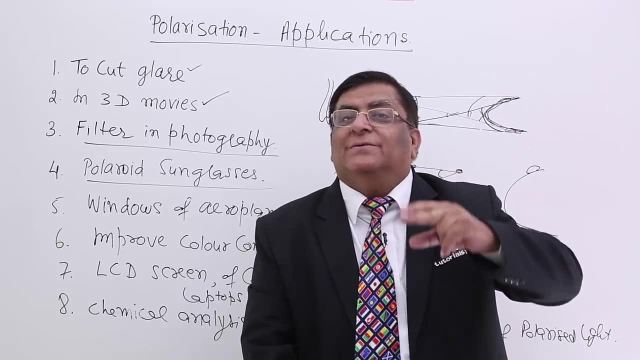 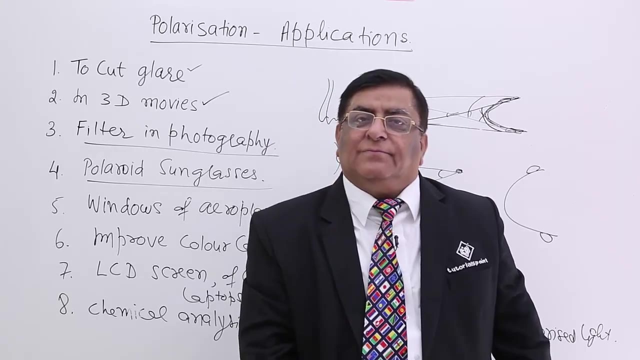 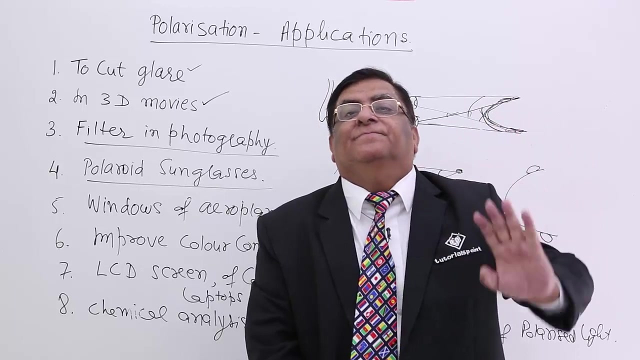 That is the problem with our colored glasses. But if we have polaroid glasses it will allow all the seven colors. What it will cut? It will cut one side of vibrations, So the total intensity Become half, and in place of sun the things appear to us as if they are placed in shade. 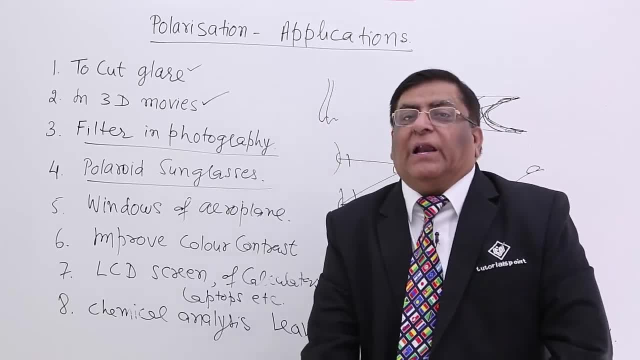 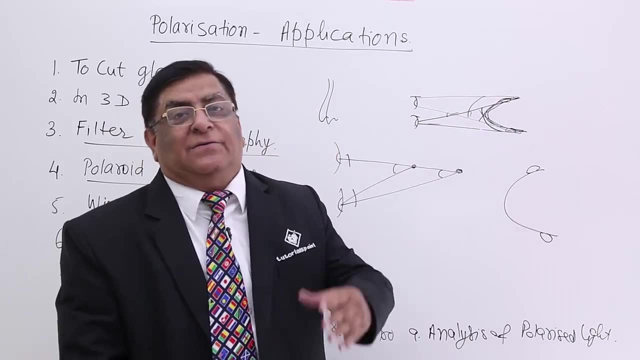 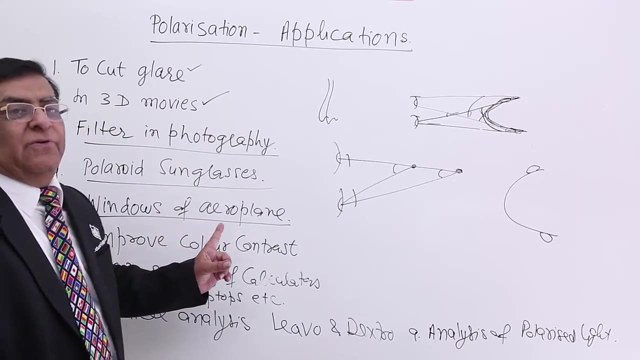 So that gives a very soothing effect. So the polaroid glasses are better than ordinary sunglasses Because they do not give any type of color defects. Then windows of airplanes: we use it So that it will cut the light. Then windows of airplanes. 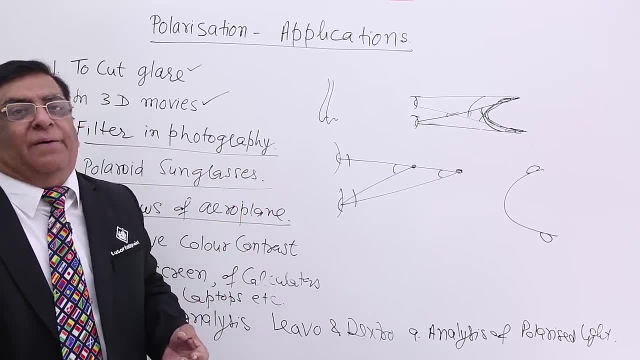 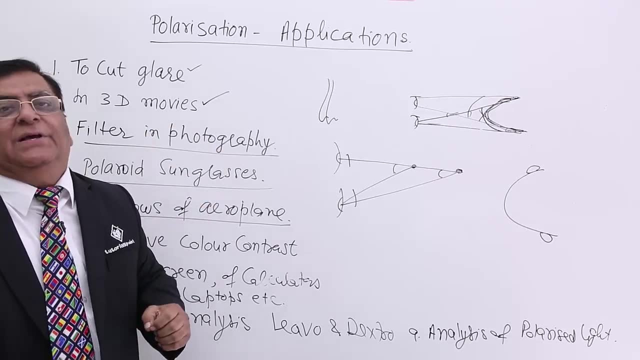 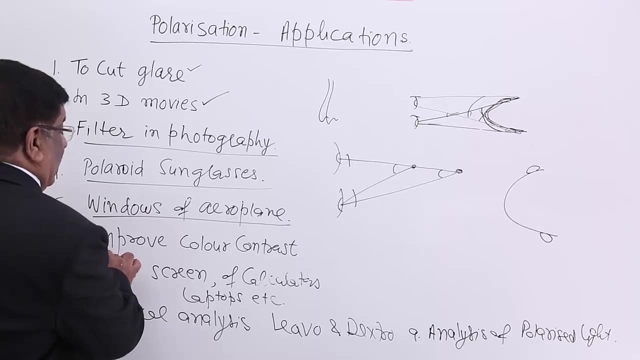 We use it And that light may also be damaging, because at the height there are ultraviolet lights, There are more powerful lights and we want to cut that glare. So we use it in the windows of airplane. Then it is also used to improve the color contrast. 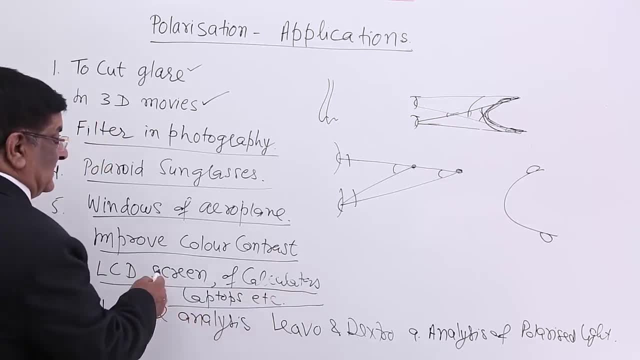 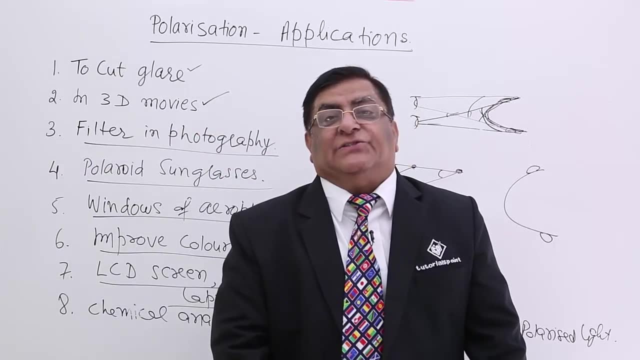 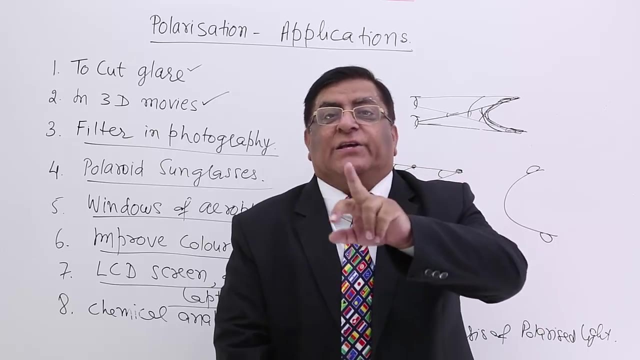 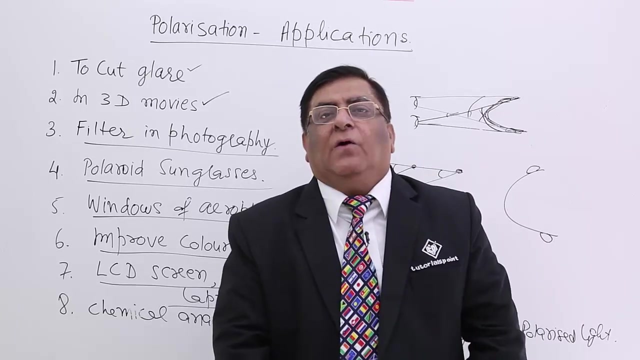 In the pictures. it is also used in LCD screen. If you have studied about LCD, LCD TV, LCD screen In our laptop, LCD in our mobile or in our calculator, specially calculator, What happens in that? how those black figures appear? Whenever we press a button, that particular area becomes a little hot. 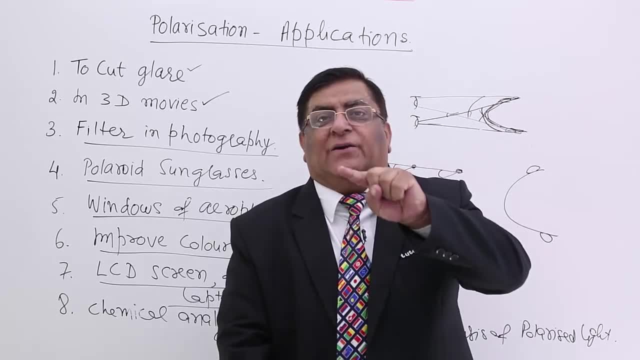 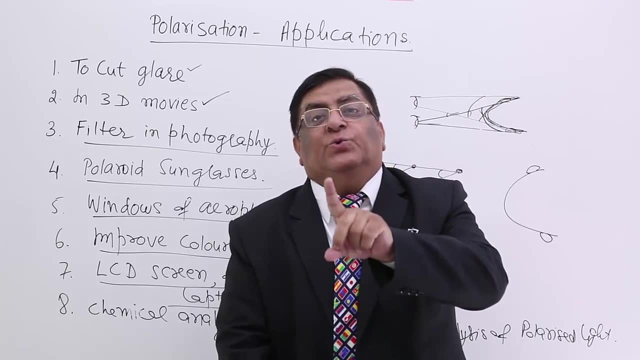 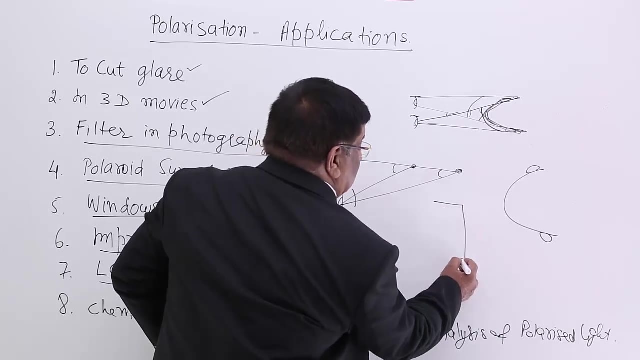 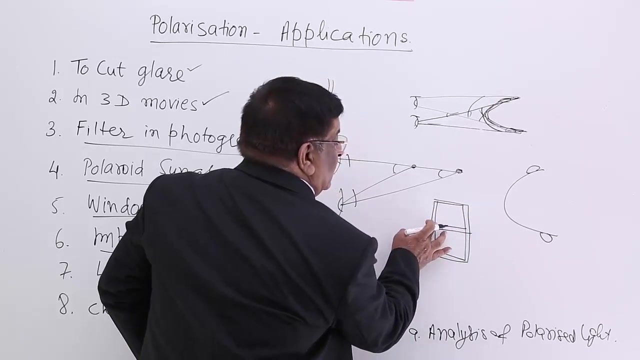 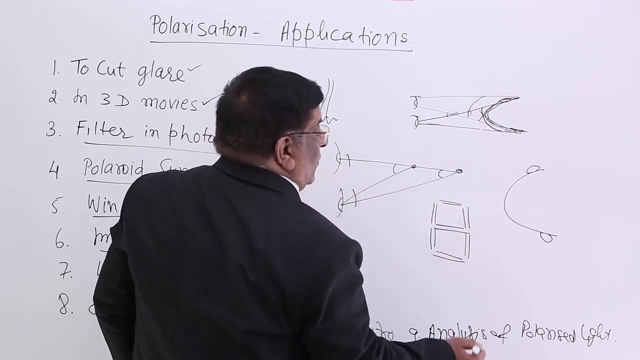 When that becomes hot, the chemical there convert into light. Sorry, Chemical there which was solid convert into liquid. What it has become? Liquid crystal. So if there is, these are the crystals. You know there are 8 crystals like this. Yes, this way. 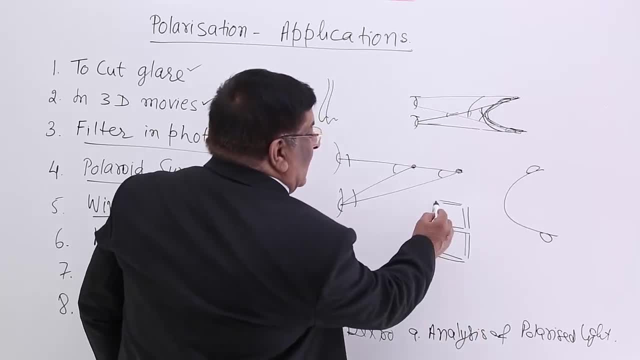 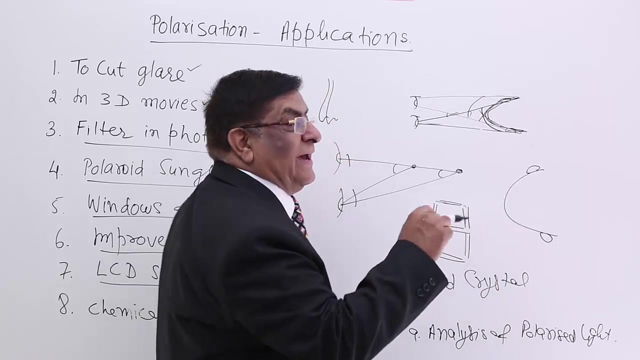 So if you switch on 8. The current will go In all these 8 crystals. What will happen? They because of that current. they will become liquid, Liquid crystals. When they become liquid, what happens? Answer is: when they become liquid, they become polaroids. 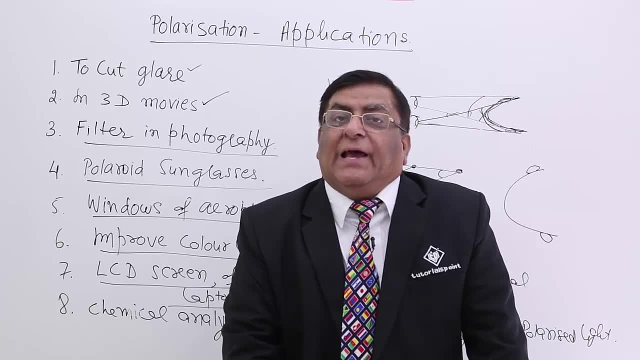 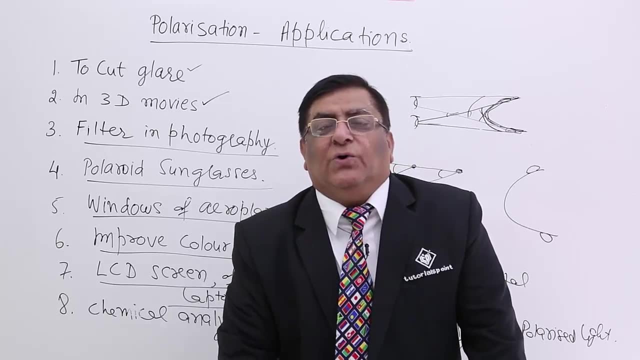 Their construction is such that they become polarized. And when they become polarized, the intensity of light coming through them is cut. So if they become liquid, They become polaroids, They become polaroids. If the light is not coming from this place, how it will appear black?